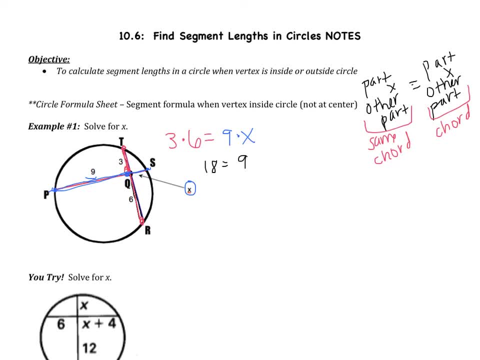 3 multiplied by 6 is 18.. 9 multiplied by x is just 9x. If I divide by 9,, I get x equals 2.. That's it. So you just have to remember to look at one chord at a time and then compare it to another chord. 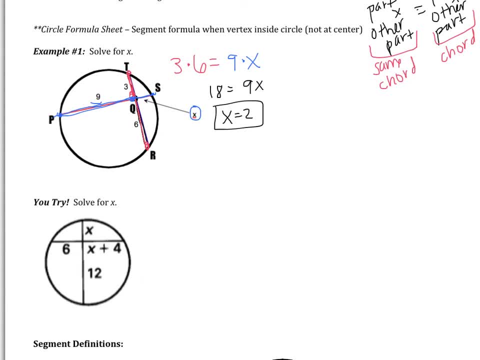 Okay, time for you to try Pause the video and try this one on your own, please. Good luck. Okay, I will tell you. you should have gotten x equals 4.. When you come to class tomorrow, I will be checking to make sure that you have the work and the correct answer for this problem. 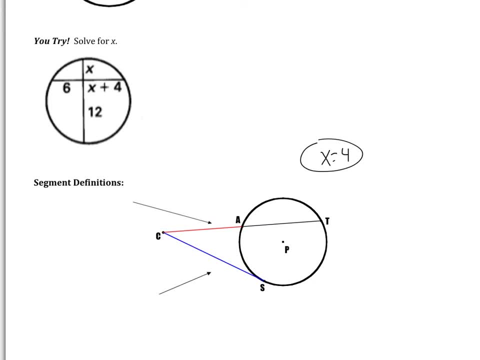 So we're going to move on to some definitions. First, looking at CT, This is a secant because it intersects a circle in two spots, once at A and once at T. This part that's outside of the circle is called the external secant. 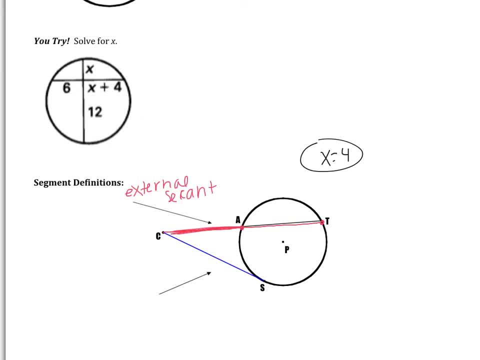 So it's the secant, but it's the part outside the circle And then CS. you should already be able to label that because we learned that in the first section. It's a segment intersects the circle once this is called a tangent. 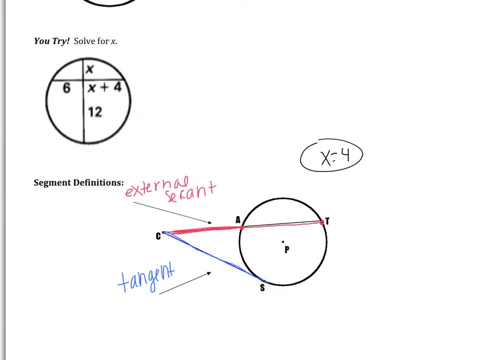 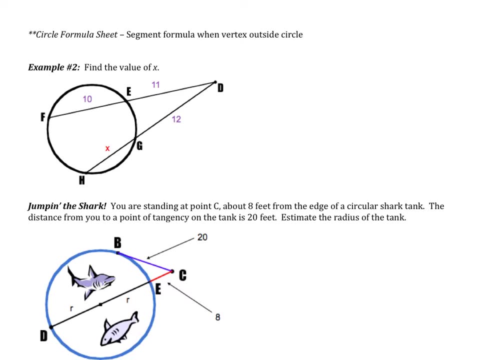 That's just a little vocab for you. If you flip the page, we're now going to jump to our next formula. Okay, So this formula is the segment formula when the vertex is outside of the circle. So the formula for this one is: outside times whole equals outside times whole. 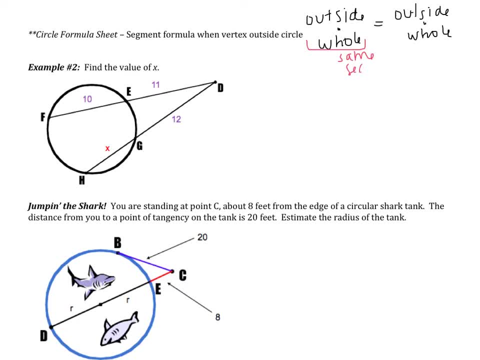 This comes from the same segment. This also comes from the same segment. Okay, Again, very vague formula, so let's just illustrate it. Looking at example two, it says: find the value of X. Well, our vertex is outside the circle D. 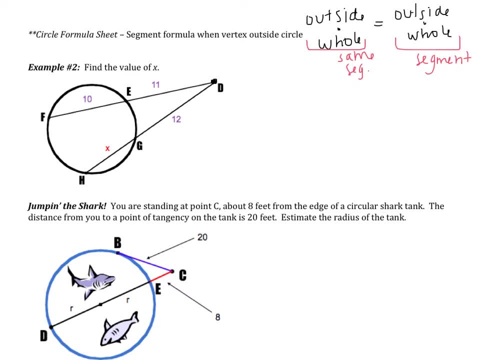 So I need to look at one segment at a time. I'm going to start by looking at segment FD. Okay, So it says outside that's this part, the external secant part. So it's going to be 11 multiplied by the entire segment. 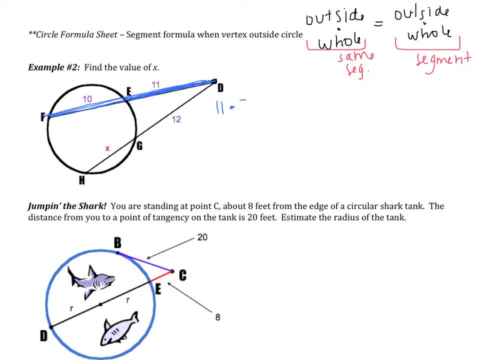 So that's all of FD. So that's going to be 10 and 11.. Which is 21.. Equals. now I'm going to look at my second secant. Okay, So the formula says outside again, which is the GD part 12, multiplied by the entire. 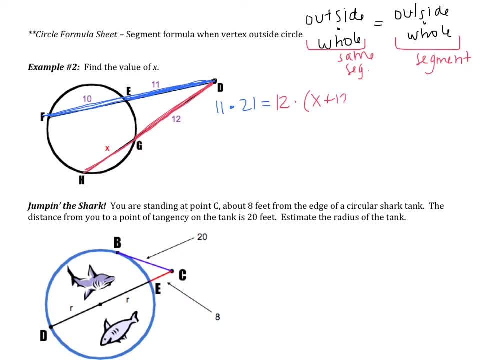 segment HD, which is going to be X plus 12.. And then I need to simplify. Okay, So solving the left side becomes 231, equals the right side becomes 12X plus 144.. If I subtract 144, I get 87 equals 12X. 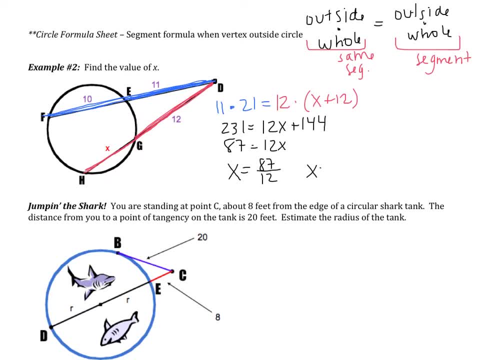 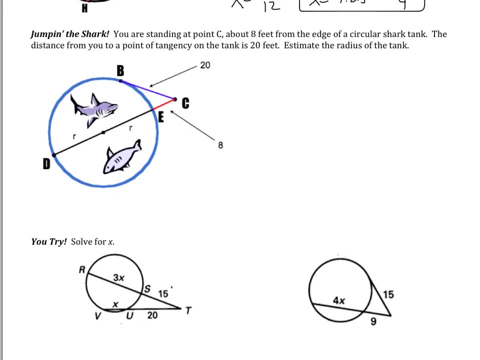 So X equals 87 divided by 12.. That simplifies to be 7.25, which is the same thing as 29 over 4.. Okay, So let's look at another example. We're going to do one more together, and then you're going to do two on your own. 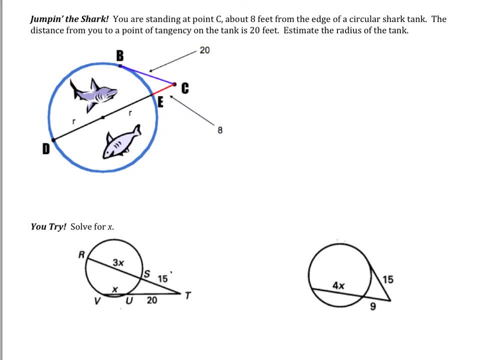 So this next one. it's called jumping the shark. It says You are standing at point C, about 8 feet from the edge of a circular shark tank. The distance from you to a point of tangency on the tank is 20 feet. 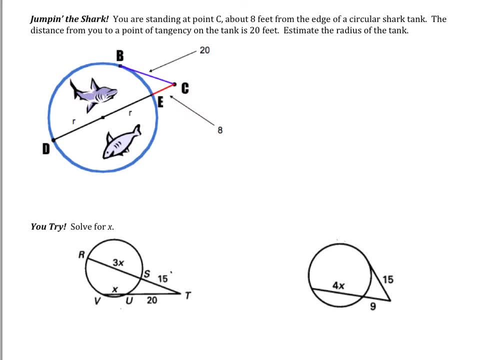 Estimate the radius of the tank. Okay, So you're standing at point C. You're standing at a point outside of the circle. The vertex of the angle is outside of the circle, So it's going to be part outside times whole. equals outside times whole. 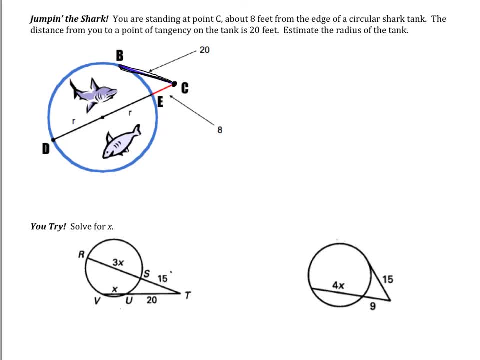 Let's look at our first segment, The BC. The part that's outside is 20.. And then the whole is still 20.. That's because this segment is a tangent. So anytime that the segment is a tangent, you're just going to be using the same segment twice. 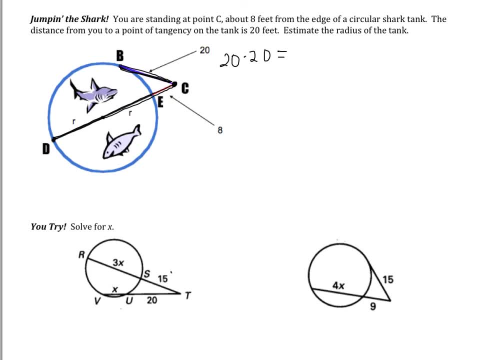 Now let's look at our other segment. This is a secant. Okay, In this case the outside part is right. here The outside part is 8.. And then this DC is the entire segment. So that's going to be 8 plus R plus another R. 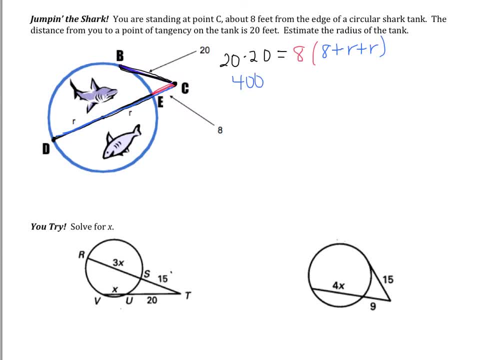 Okay, On the right side this becomes 400. I mean on the left side 400.. Right side it's 8 multiplied by 8 plus 2R. When I distribute that 8, I get 64 plus 16R. 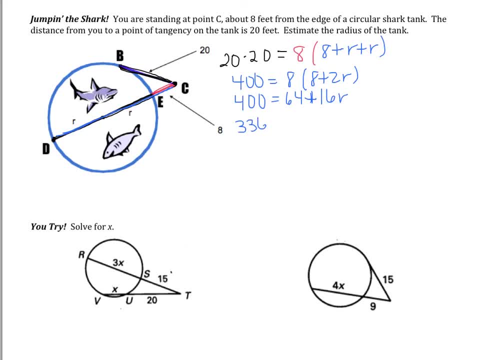 Subtracting 64, I get 336 equals 16R. Dividing by 16,, I get R equals 21 feet. So the radius of the tank is about 21 feet. Okay, Again, here are the two that you're doing on your own. 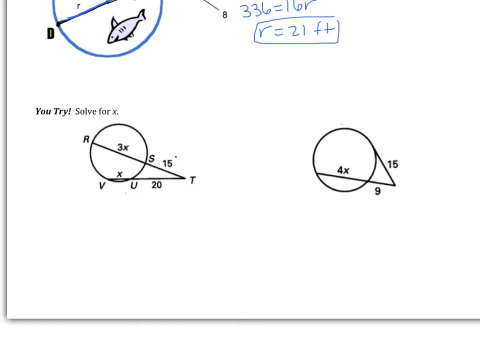 I would like you to pause the video and do both on your own, please. Good luck. Okay, Let's see how we did In the first example, vert. Sorry, Vertex is outside the circle, So I'm going to do outside times whole. 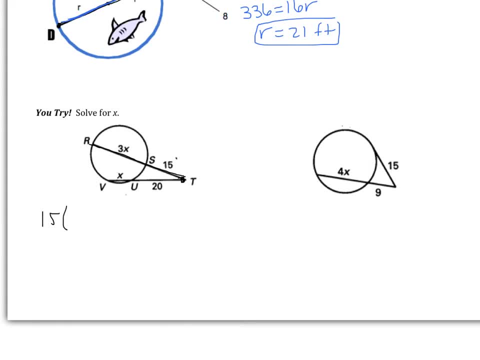 Looking at the first secant, the outside part is 15.. The whole is going to be 15 plus 3X. Looking at my other secant, the outside is 20.. The entire is 20 plus X Distribute on both sides. 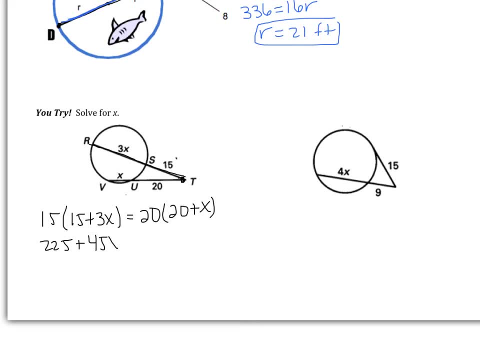 I get 225 plus 45X equals 400 plus 20X. If I subtract 20X, I get 25X, equals Subtracting 225 from 400, I get 175.. So then I have X equals 7.. 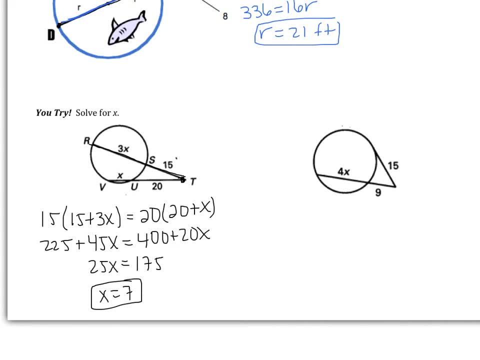 Hopefully that one went well for you. Now for the second example. you should have gotten X equals 4.. If you didn't, you need to go back and find your mistake. When you come to class tomorrow, I'm going to be making sure that you have all the work completed with the correct answer. 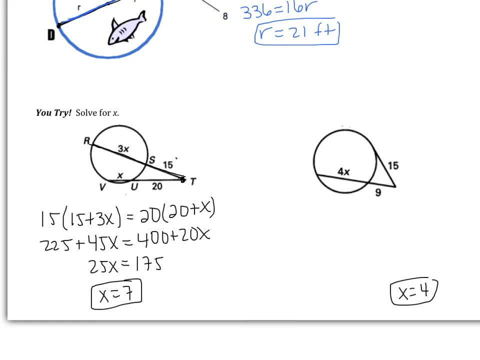 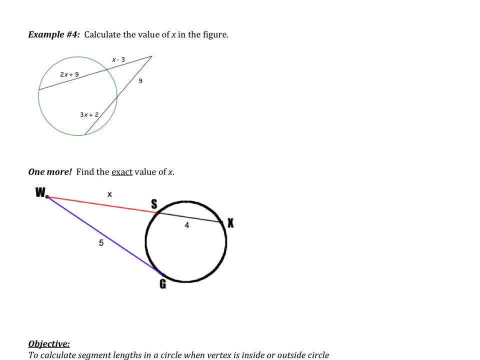 If you have any questions, feel free to ask tomorrow. Now let's flip to the next page. Okay, So we have two more. These are definitely two more difficult examples, So we're going to do them together. They're not difficult because of the setup, but difficult because of the solving. 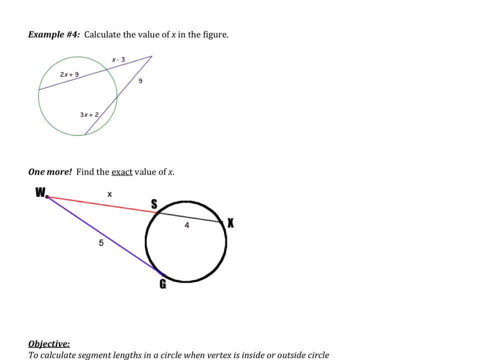 Example number four says: calculate the value of X in the figure. Okay, I have my vertex outside the circle, So it's going to be outside times whole equals outside times whole. Looking at my first secant, the outside is X minus 3.. 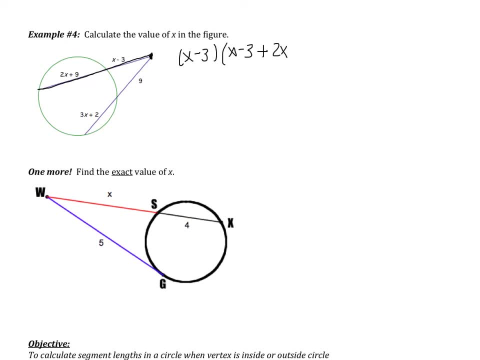 The whole is X minus 3.. Add 2X plus 9.. Right side or the right secant. the outside part is 9.. The entire part is 9 plus 3X plus 2.. Okay, Simplifying the left side. X minus 3 cannot be simplified. 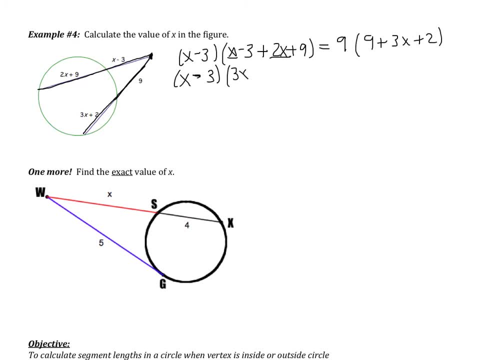 I have X and 2X, which is 3X. I have negative 3 and positive 9, which is going to be positive 6.. On the right side I have 3X plus 9 combines with 2 to become 11.. 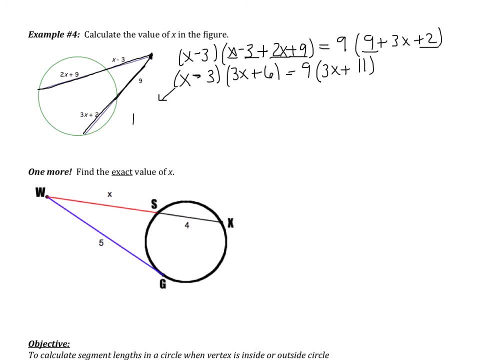 Okay, Now here's where I'm going to have to draw a box to multiply these- Or some of you use that other term that I'm not going to say- 3X and X is 3X, squared 3X and negative 3 is negative 9X. 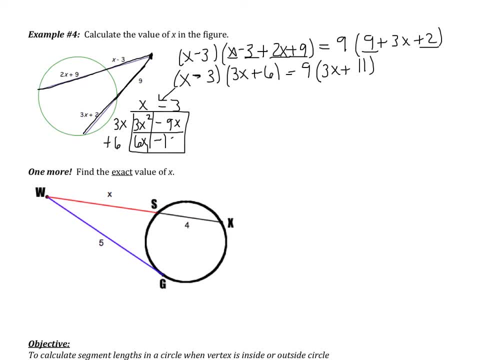 6 and X is 6X 6 and negative 3 is negative 18.. So the left side really is 3X squared, And then negative 9X, positive 6X becomes negative 3X, Then I have minus 18 equals. 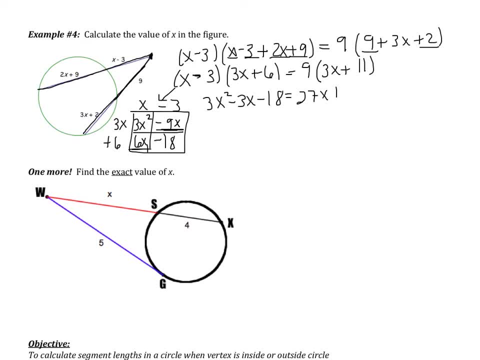 When I distribute the 9,, I get 27X plus 99.. Okay, I'm going to move everything over to one side. So that means subtracting 27X, subtracting 99.. So I have 3X squared minus 30X minus 117 equals 0.. 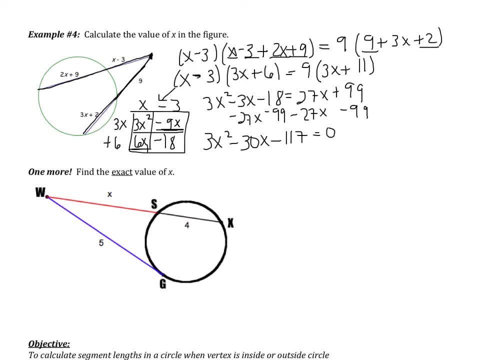 Okay, Any time that you have an X squared and an X you're going to have to factor. I'm going to start by factoring out a 3.. Everything here is divisible by 3.. When I factor out a 3, I get X squared minus 10X minus 39 equals 0.. 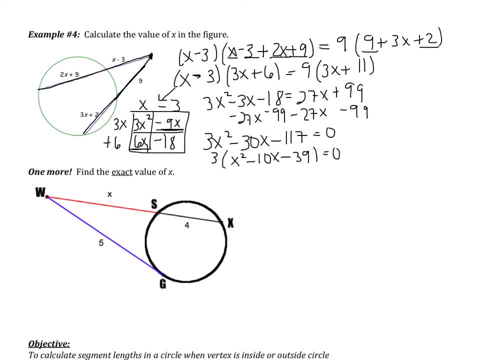 This is going to make my factoring a lot easier, since I was able to factor out a 3.. Now all I'm looking for are two numbers that multiply to negative 39 and add to be negative 10.. The only factors of 39 are 1 and 39,, which certainly don't add to be 10,, and 3 and 13.. 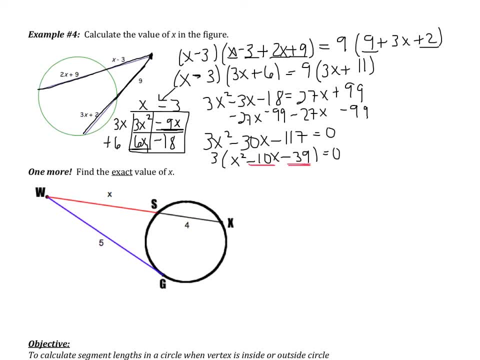 That sounds better. Positive 3 and negative 13 are going to add to be negative 10.. So this factors to be X plus 3, X minus 13. And it's still set equal to 0.. Now I set both equal to 0.. 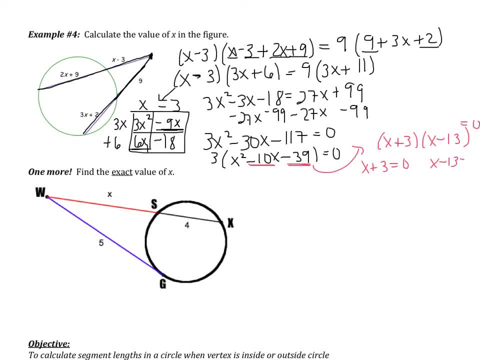 So X plus 3 equals 0. X minus 13 equals 0. I get X equals 13.. X equals negative 3.. Now, looking at my figure, I need to make sure that both make sense. Well, when I substitute in negative 3,, I have negative 3 minus 3, which is going to be negative 6.. 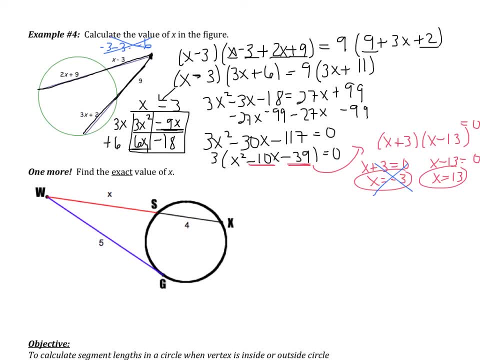 It does not make sense to have a segment that's negative 6. So negative 3 is not going to work. Our only answer is going to be positive 13. So this was a little bit of a review of factoring. 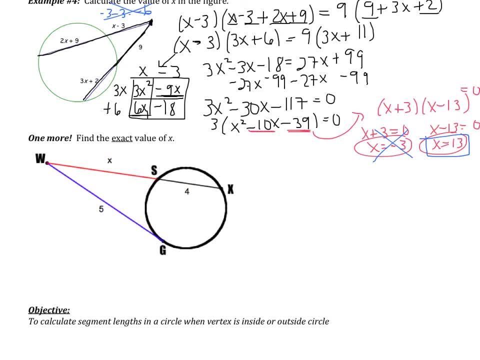 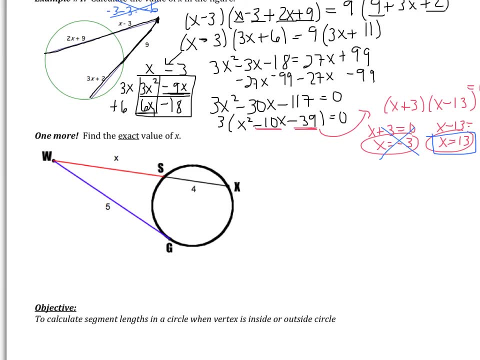 Hopefully it jogged our memories a little bit. The next example we have is also going to jog our memories, So prepare yourself. So in this case, we have a secant WX and we have a tangent WG. 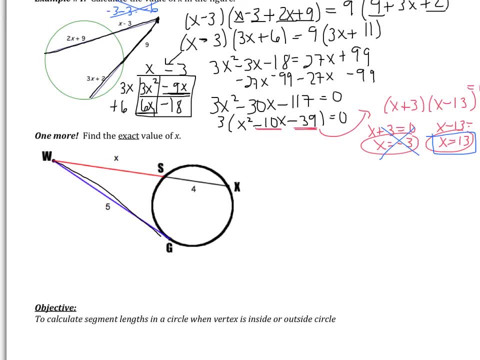 Looking at our tangent first, the outside is 5.. The whole is also 5.. Looking at our secant, the outside is X, The whole segment is X plus 4.. So I have 25 equals X squared plus 4X. 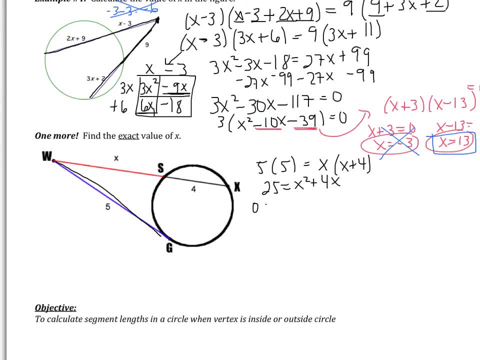 If I move the 25 over, so I subtract 25, I have 0 equals X squared plus 4X minus 25.. Okay, so again we have an X squared and an X term, so we need to try to factor. 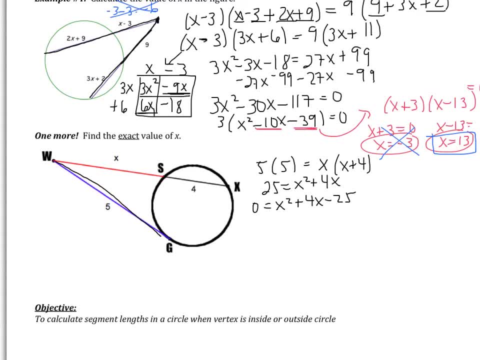 So I need to think what two numbers multiply to negative 25, but add to be 4? Well, the only numbers that multiply to 25 are 1 and 25, or 5 and 5.. Neither of those cases add to be 4.. 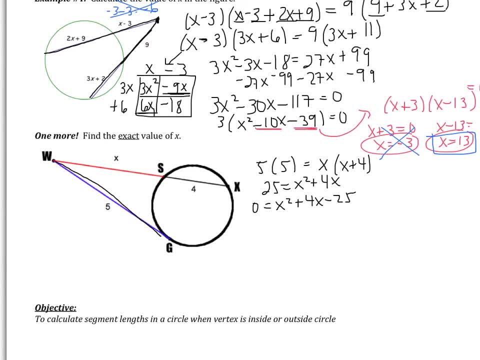 So this does not factor. We have to use the quadratic formula. So hopefully you remember the quadratic formula. If not, I'm going to write it down. You probably learned a song for the quadratic formula last year. I'm not the best singer, but in order to help us, I will sing it for us. 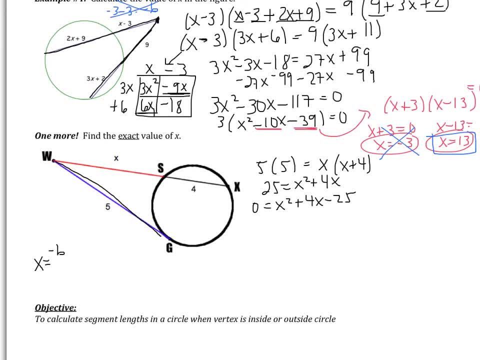 So we have: X equals the opposite of B, plus or minus the square root, B squared minus 4AC, all over 2A. That was supposed to be Pop Goes the Weasel. I understand, my voice is not that good, But this is the formula. 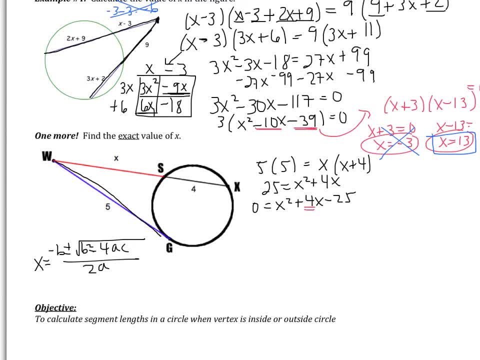 So B squared minus 4AC, B is what's in front of the X term, A is what's in front of X squared and C is the last term. So in this case, if B is 4, the opposite of B then is going to be negative 4. 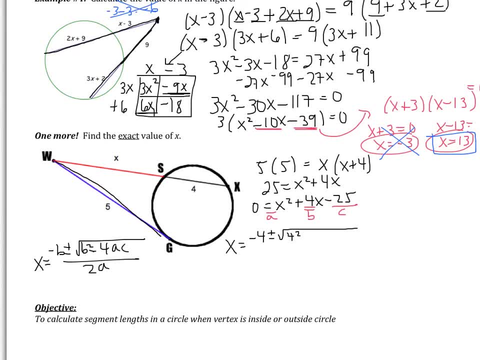 plus or minus the square root of B squared, so 4 squared minus 4 times A, times C, all over 2A. In front of the X squared there's not a number, so it's understood to be a 1. Okay. 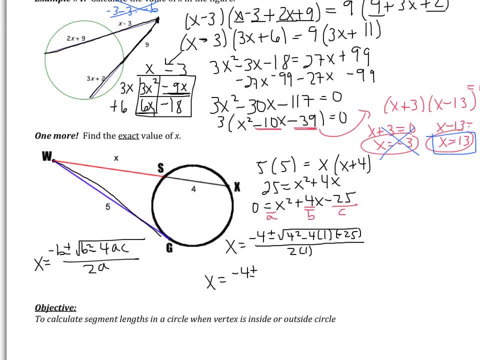 Now we've got to simplify. I have: X equals negative 4 plus or minus the square root, 4 squared is going to be 16.. Negative 4 multiplied by 1, multiplied by negative 25 is going to be positive 100.. 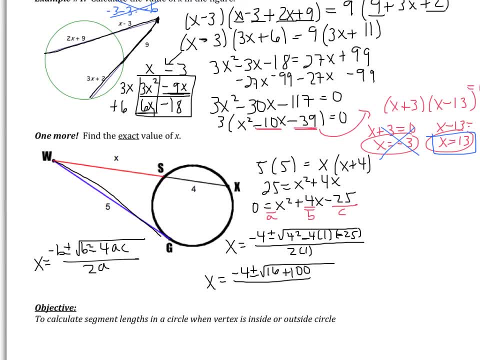 That's because I have this negative 4 and the negative 25.. This is all over 2.. Okay, So this is negative 4 plus or minus the square root of 116, all over 2.. Before I do anything else, 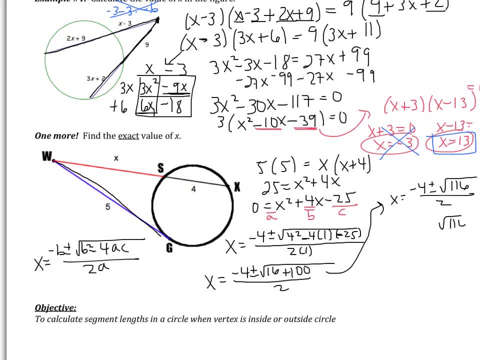 I have to simplify that: square root of 116.. So 116 is 4 times 29.. 4 is 2 times 2.. 29 is left over. It doesn't break down. So I have X equals negative, 4 plus or minus. 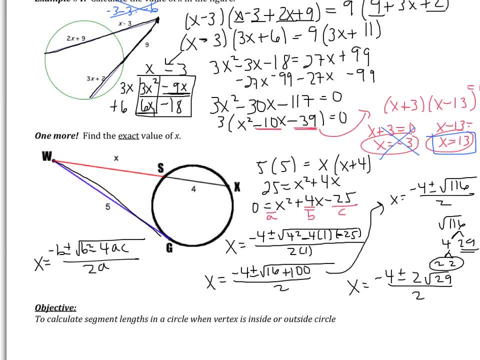 A, 2 comes out, 29 stays under the root, all divisible by 2.. Not done yet, Negative 4, 2, and 2 are all divisible by 2.. So I'm going to divide them all by 2.. 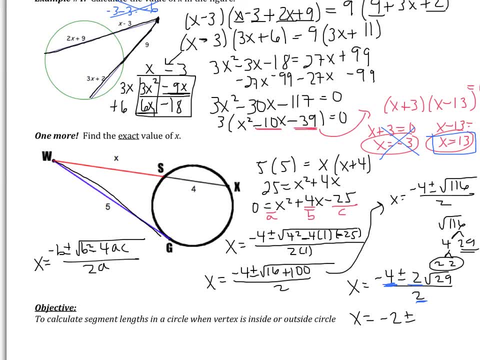 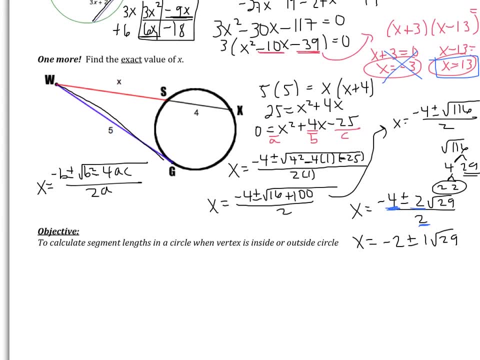 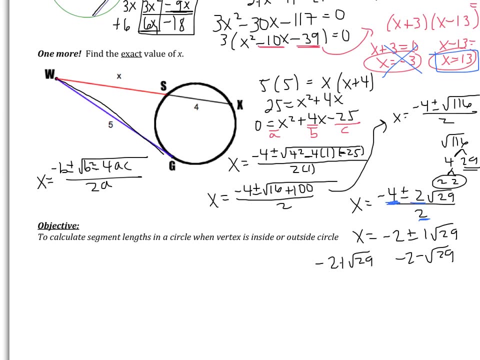 So I have: X equals negative 2 plus or minus 2. divided by 2 is just 1 root 29.. Okay, So this gives us two answers: Negative 2 plus root 29.. Negative 2 minus root 29.. 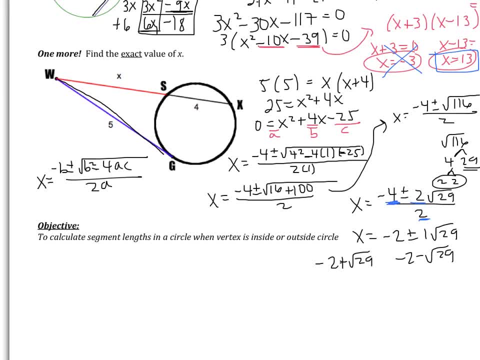 Okay, If I get decimal approximations for both of those, I get about 3.39 and about negative 7.3.. Now, looking at our figure, negative again doesn't make sense. So this is my only answer: The negative 2 plus root 29,. 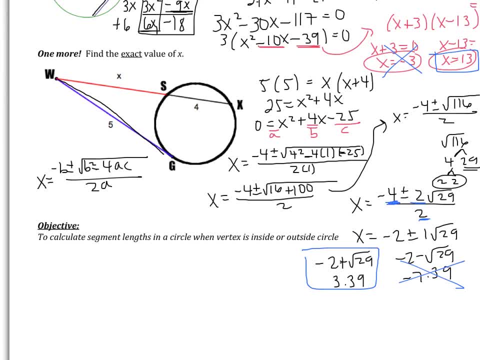 which is about 3.39.. If you don't remember this, if you don't remember the quadratic formula, that's totally fine. At a minimum, I expect you to be able to set up the problem. We will review a little bit more of this in class. 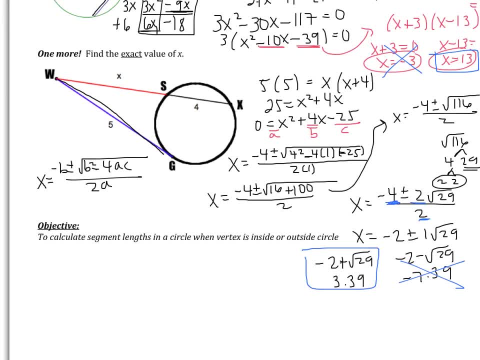 And this was just to start jogging in our memories so we can remember some of that stuff that we learned last year in algebra. That brings us to the end of our video. Today's objective was to calculate segment lengths in a circle when the vertex is inside or outside of the circle. 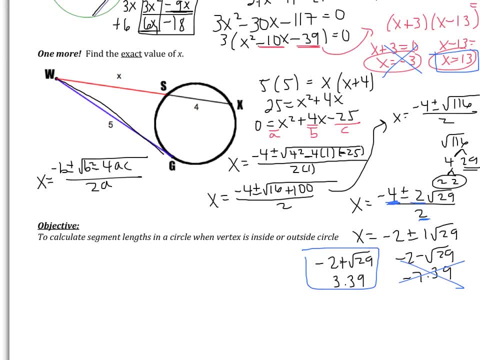 So when the vertex was inside of the circle we only did two examples. You multiplied two parts and set them equal to the two other parts When the vertex is outside. that was a little more complicated. It was: part times whole is equal to outside times whole. 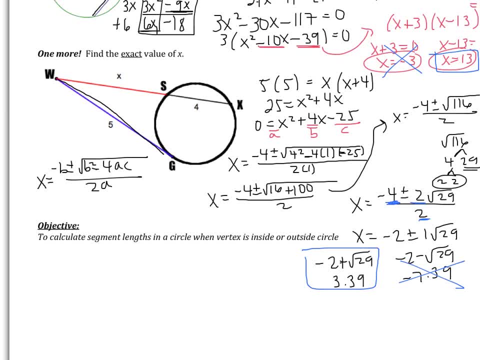 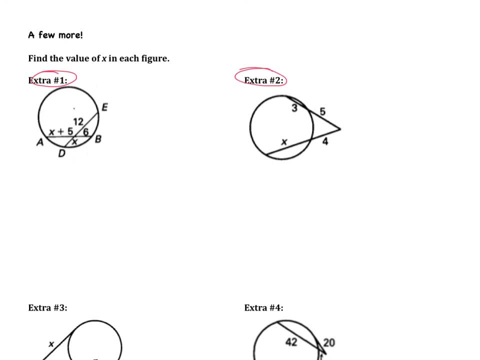 If you flip the page there's a few more examples. Okay, On this page you have two problems to do in order to get your video checked in for tomorrow. You're going to be doing extra examples- numbers one and two- When you come to class tomorrow. 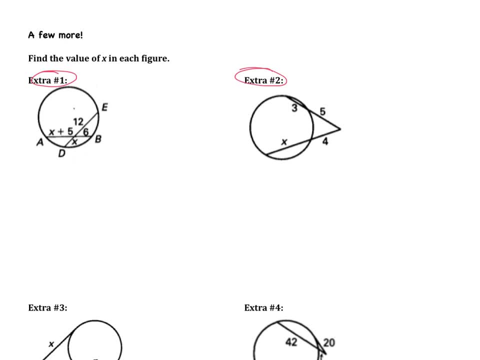 I'm going to be making sure that you have both of these problems completed with work. I will tell you the answers to both. For extra example number one, you should get x equals five. For extra example number two, you should get x equals six. 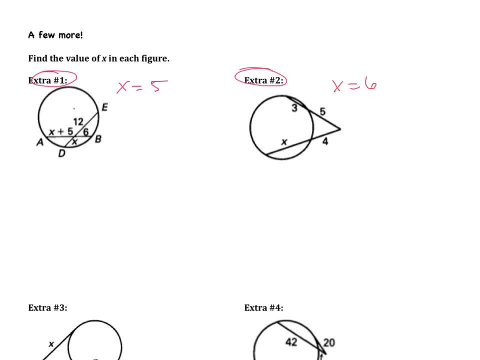 If you don't, you did something wrong. If you're not sure what to do, look back at the previous examples and the two formulas that we learned in the video. Again, when you come to class tomorrow, I'm going to be checking the entire video. 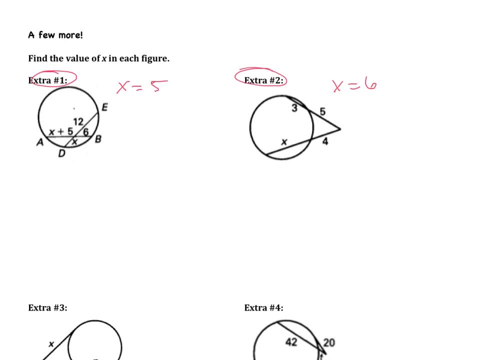 plus these two problems. Good luck, Thank you.